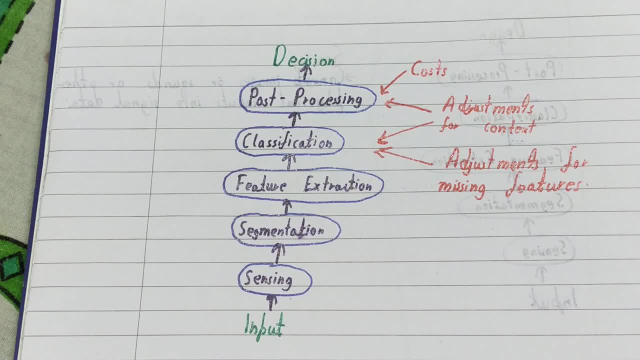 Or warm, because you're not sensing the input right. So if you are not able to sense anything, then nothing will work. Okay, so this is the most important thing. Okay, in a pattern recognition system, that is a sensing. So now let's discuss about the sensing part. So, in the sensing part, it has a particular sensor. and what a sensor does? a sensor converts images or sounds or other physical inputs into a signal data. Okay, so 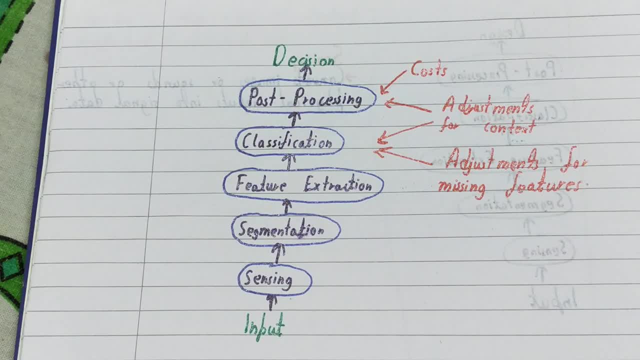 sensor receives some images or some sounds or some other physical inputs from its sensors and that particular sensor sense and it converts into into a digital form, or you can see in the form of signal data. okay, that that is readable by a computer. okay, the input to a pattern recognition system is often 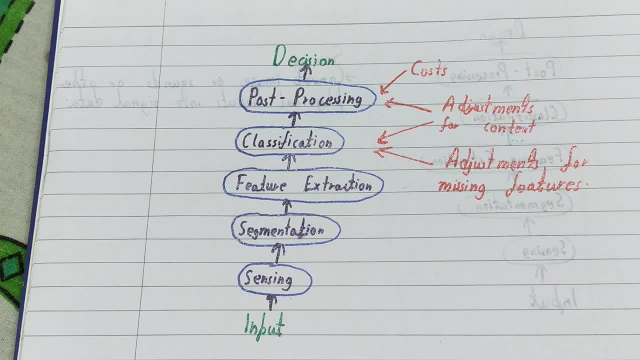 some kind of transistor. what it says is like: whatever input you are getting, whatever input the pattern recording system is taking, it is taking to a particular sensor right. so that is a kind of transducer. that particular have some limitations. for example, you are clicking a photo with your camera, right? 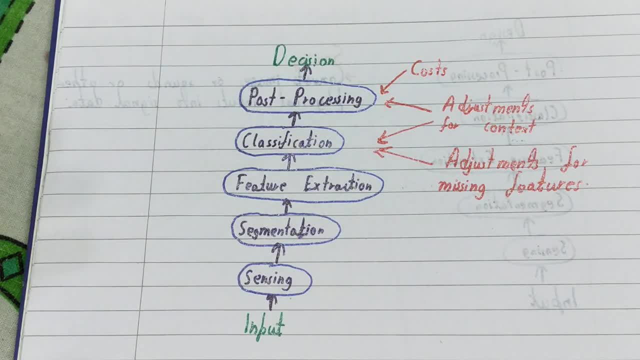 so your camera also has certain limitations. it cannot be unlimited or it cannot be fully perfect, right? so that is what it tells. okay, the quality of a pattern recognition system highly depends upon the sensor also. okay, so this is what I meant to say over here. okay, so I guess you are. 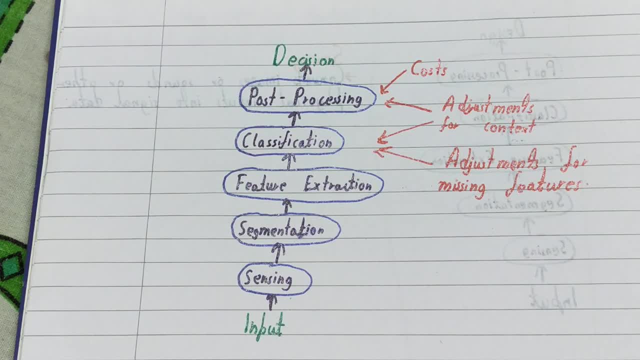 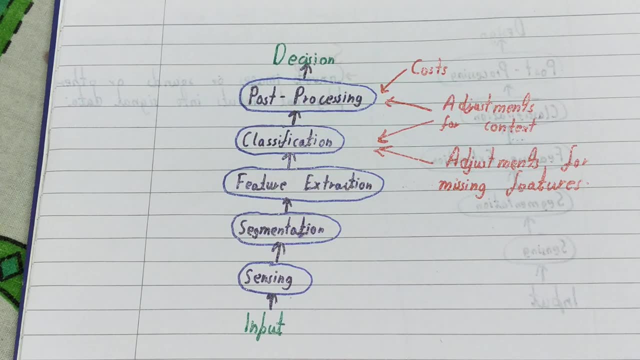 clear with the sensing part. now let's move on to the second part, that is, the segmentation part. okay, so in segmentation part, what we do is segmentation refers to a process of partitioning our digital image or speech into a multiple segments. okay, so what it says is: whatever digital data we 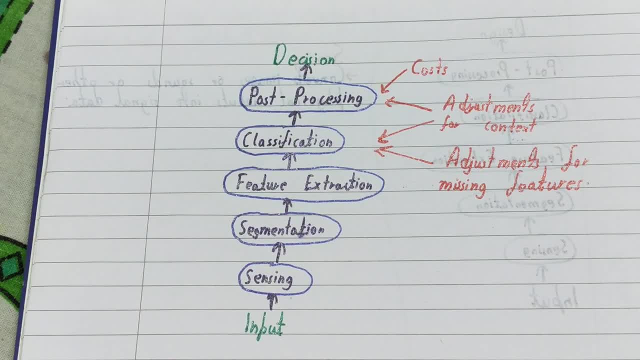 get from sensing part. we segment it into a small, small pieces, or you can say small, small processing data, so so that a computer can easily process it. okay, and also a special function is done by the segmentation part. what it is the segmentation part does a particular function by which it isolates sensed object from the background or from other. 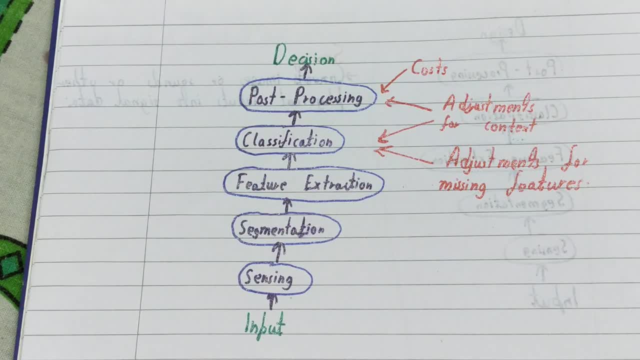 objects. so what it says is like: the important, or you can say, the data that needs to be sensed, okay, only that data is, uh, carried forward to the next stage and the rest data is left behind. okay. so again, let me give you a good example so that you'll be better able to. 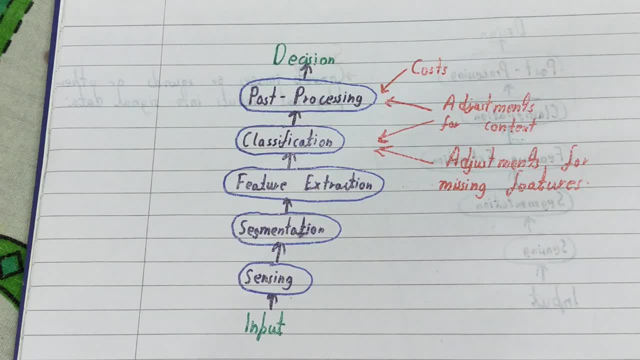 understand it okay. so, for example, same example, okay. for example, you are asked to see a particular image, right? so when you will see that particular image and you are asked to detect that particular objects like apple is kept in front of you and asked to tell that how it look like, right? 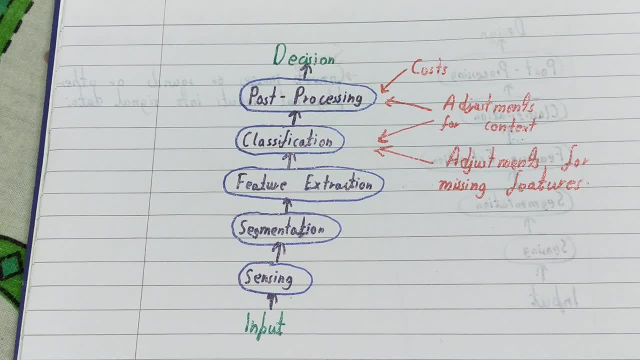 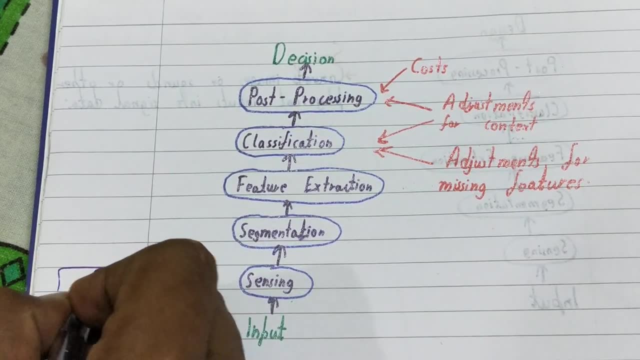 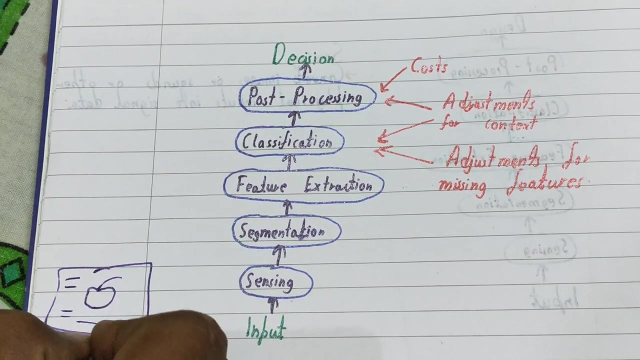 so you you will not be seeing that particular apple. you will be also seeing the other details, like on the side of apple. the apple is contained in a tray right, like let me draw apple for you. my drawing is not that good, so you will be seeing these background details also, right? 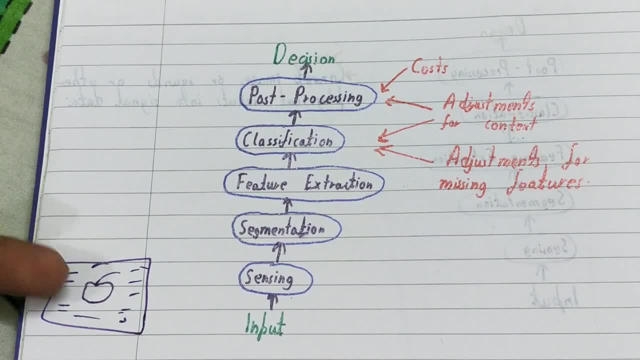 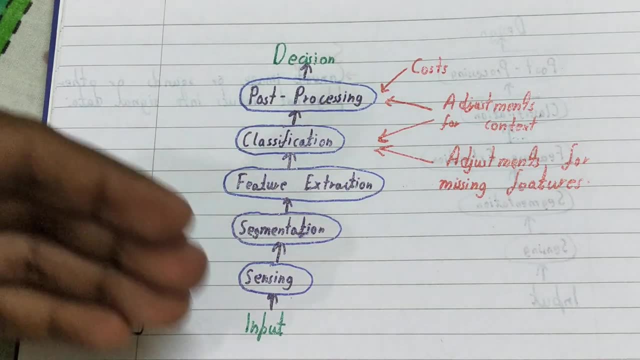 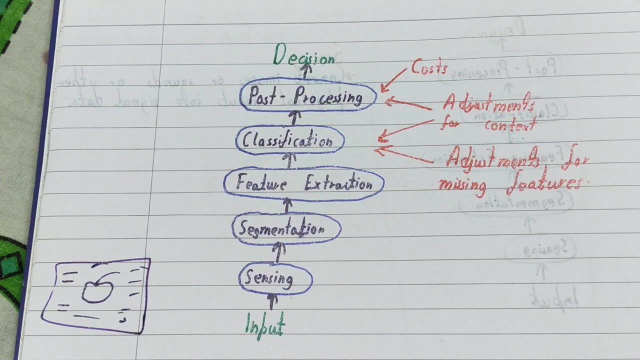 but this is not important, this is useless, right? you just need to sense this particular apple, right? so what segmentation part does first? it partitions that whole data into small, small- uh, you can say- pieces, so that it could be processed by a particular- uh- computer. or you can say the processor. 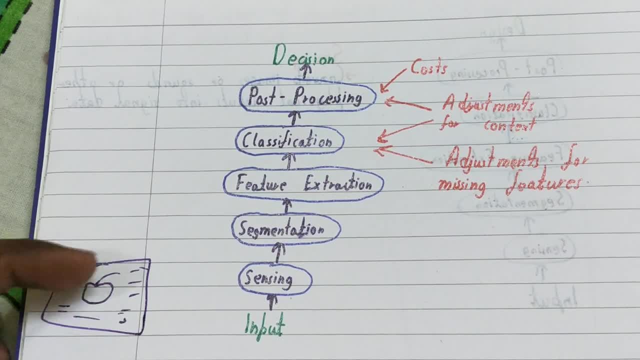 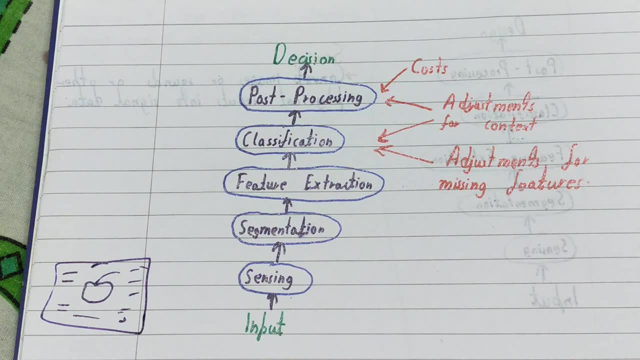 and also it only forwards the sense data, the important data, and all the left behind data is left behind, or you can say it is not forwarded to the next component, or you can say the next stage. okay, now let's discuss about the feature extraction process. so in the next stage, that is, feature extraction. 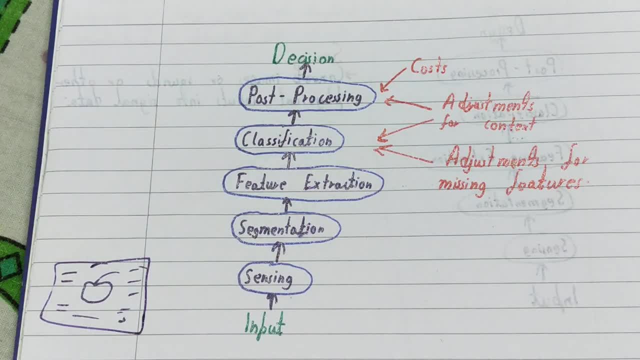 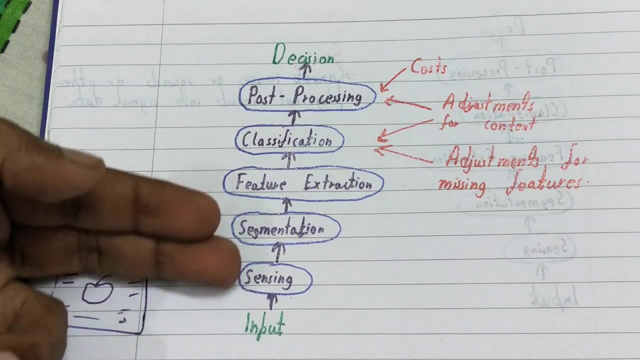 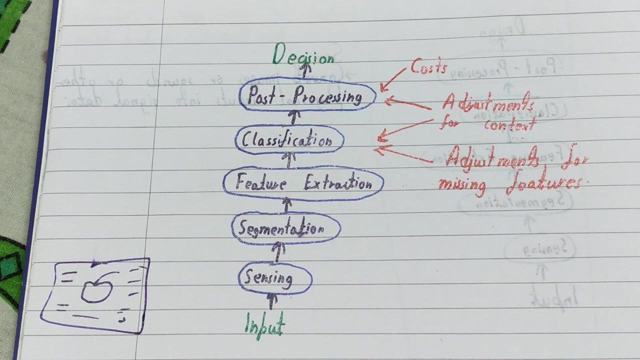 stage what it does. from the name only you can make out that we try to extract the important features from a particular object. okay, so if a particular object is sensed, okay, and then it is segmented, also for a fast processing or against the optimal processing, then a particular set of features. 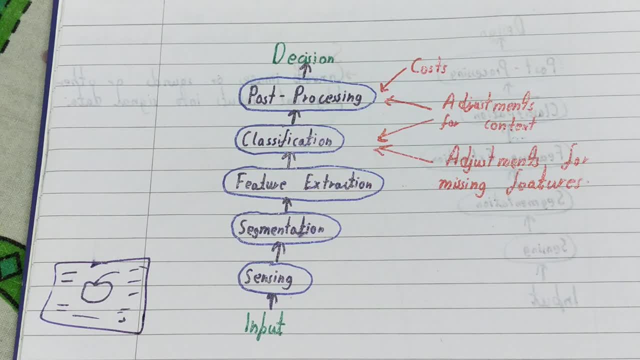 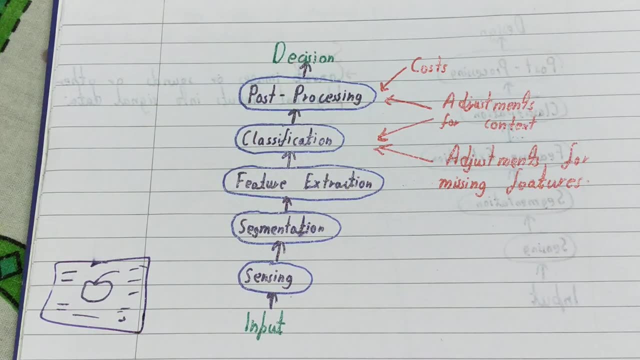 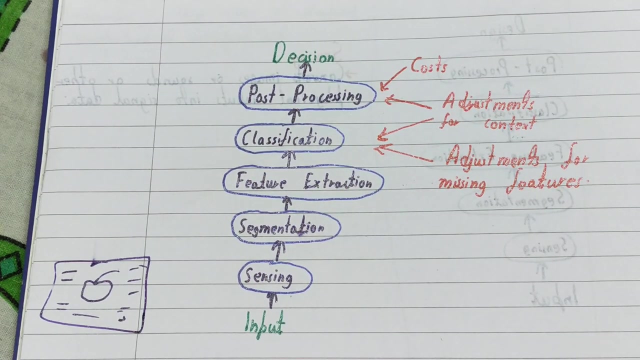 are extracted. okay, what? what features that particular object has? okay, each of the features is taken out from that particular object, so so that it could be further centered, right? so what is the work of a feature extractor? a feature extractor measures object properties that are useful for classification. okay, so, whichever property of a particular object. 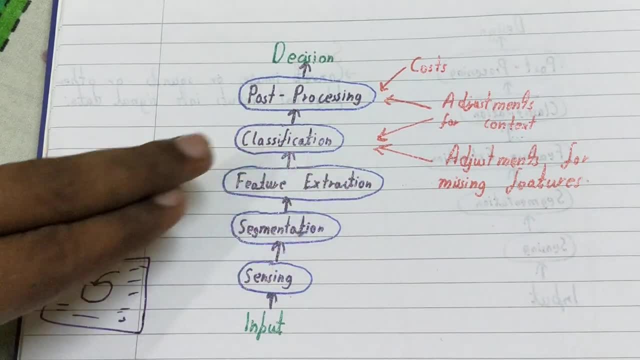 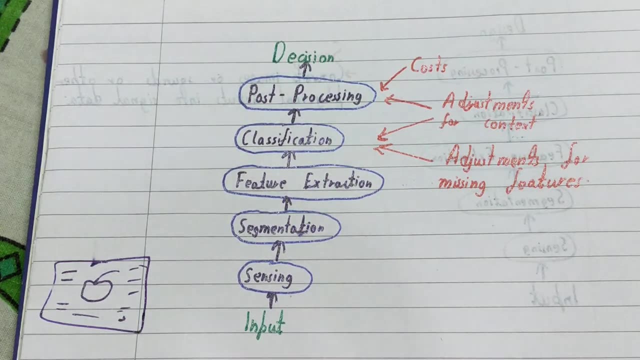 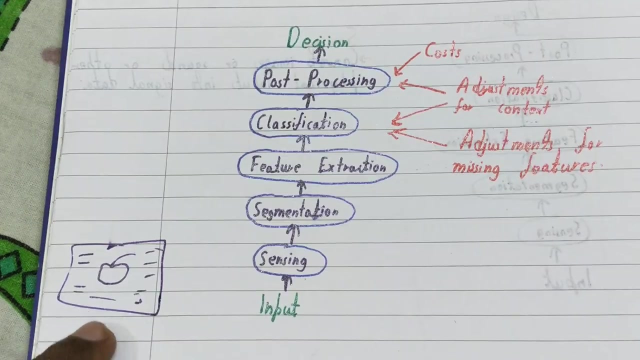 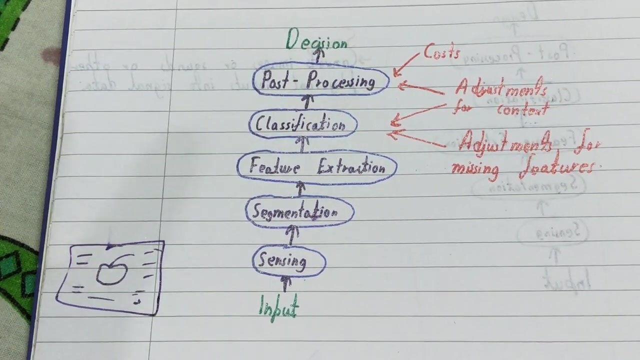 is useful for classification, that particular features from a object is classified, or you can say, is taken out. okay, and uh, the general goal, or you can say the main goal of feature extractor is to characterize an object. okay, for example, let's consider the same example, okay, of the apple, only so in this. uh, if you want, 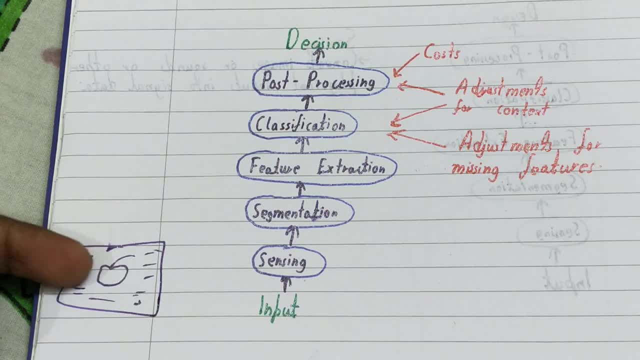 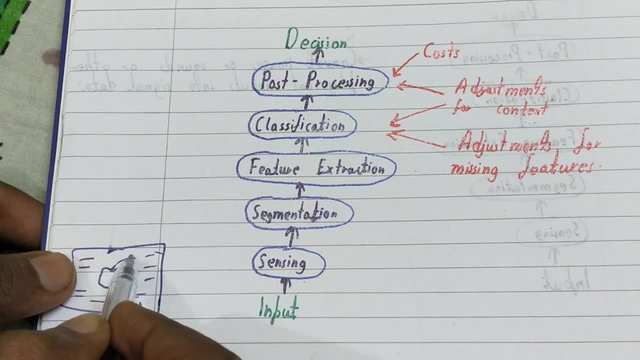 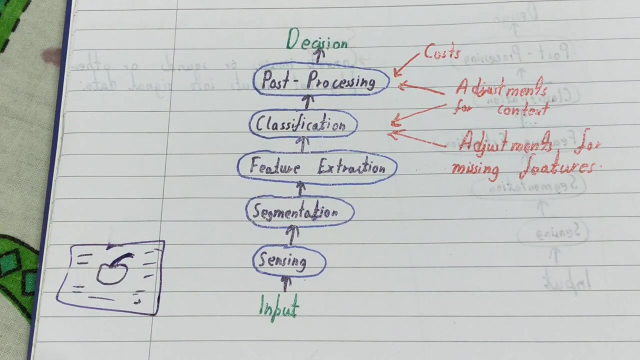 to extract a particular feature, you can see that the feature is certain, like uh, it's round shaped and from this, from here, it is curved and something- uh, uh, you can say us something is coming out from here and this looks like a right. so there are certain features by which you can tell that this. 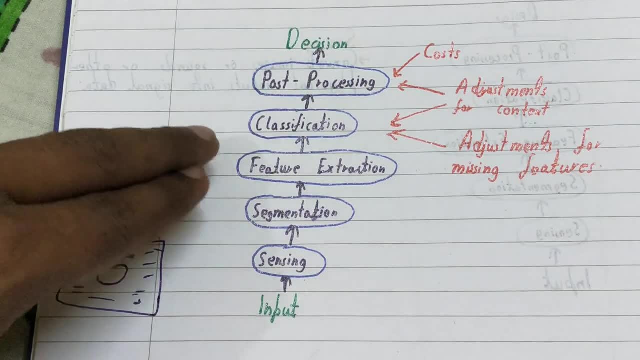 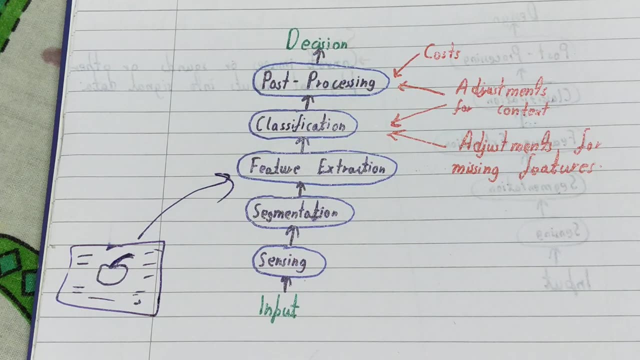 particular thing is apple, right, so that is very important in the feature extraction process. okay, so without the feature extraction process, you will be not be able to characterize a object, or you can say what, what feature a particular object has. okay, so this was all about feature extraction process. now let's move on to the classification. or you can say: the most important. 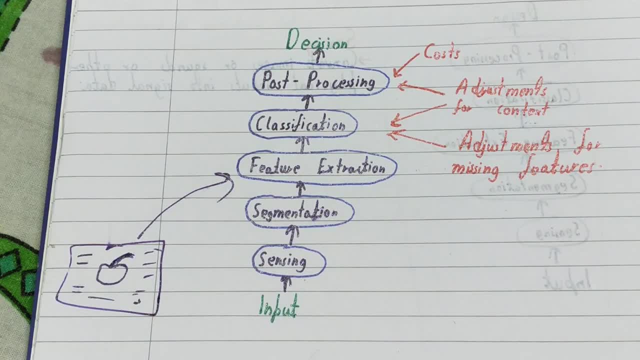 feature in the feature extraction process. okay, now, this is a very, very, very important thing in uh pattern recognition. that is the classification. so if we talk about classification, the task of a classifier, component of a full system, is to use the feature vector that is provided by the feature. 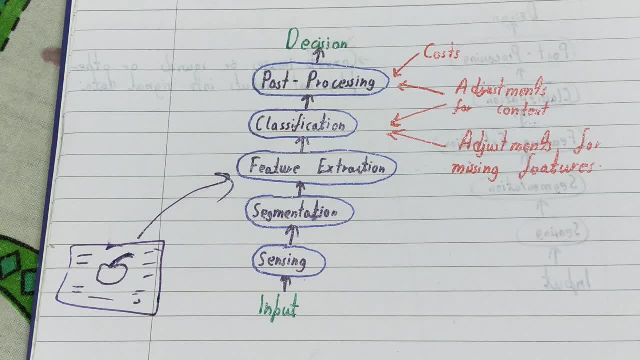 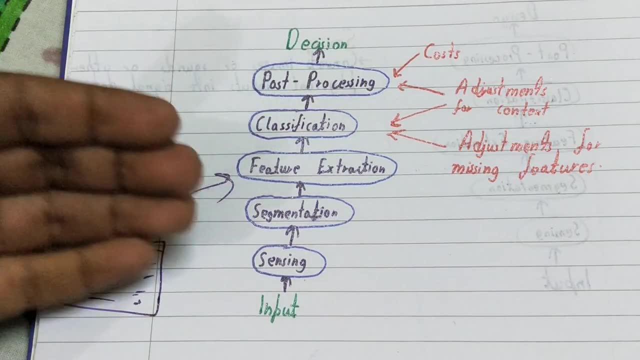 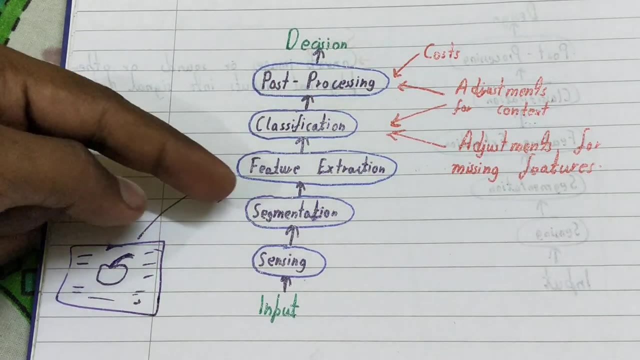 extractor and it is used to assign a particular category to object. right, so what a classifier or classification stage does is, uh, whatever and the data or whatever, the features that are provided by the feature extractor of a particular object. on the basis of that features, uh, the classification stage decides. 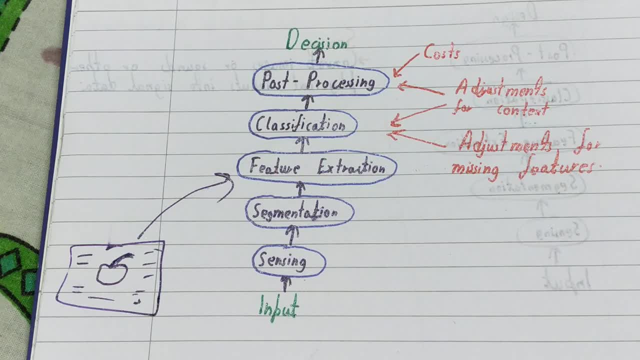 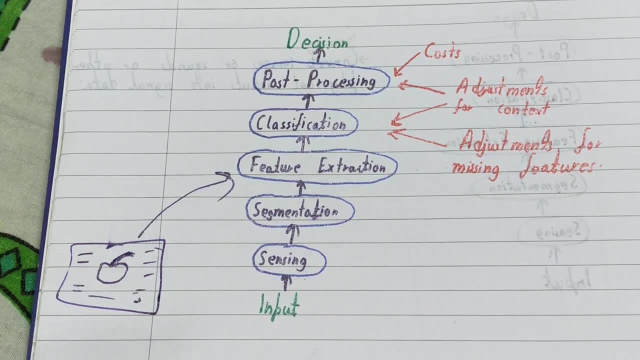 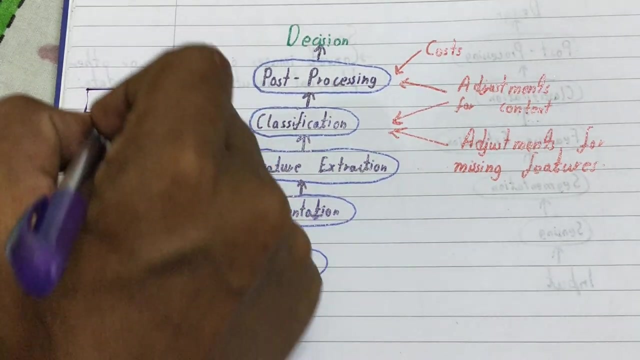 that okay, uh, this particular objects belong to this category, or this particular object is kept into a particular category, okay. second thing, on the difficulty in classification: depends upon the difficulty in the difference among different objects, uh features. for example, you are asked to detect uh different, different shapes, okay. 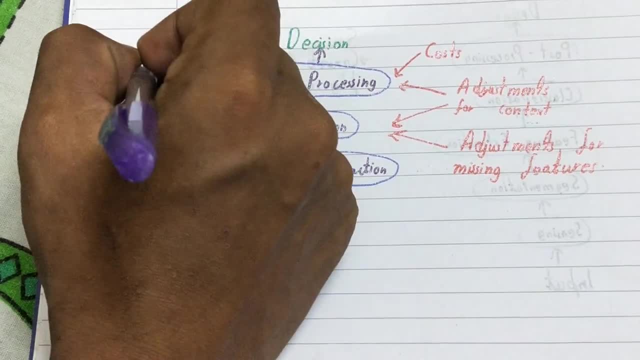 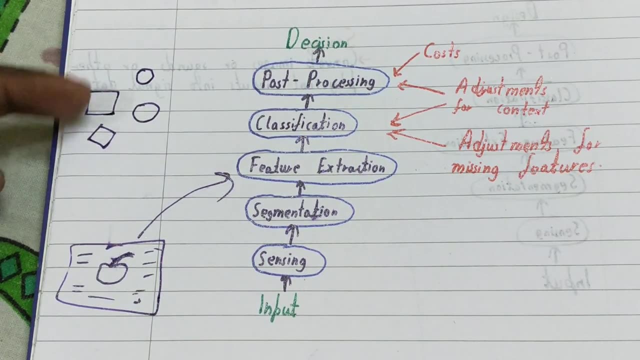 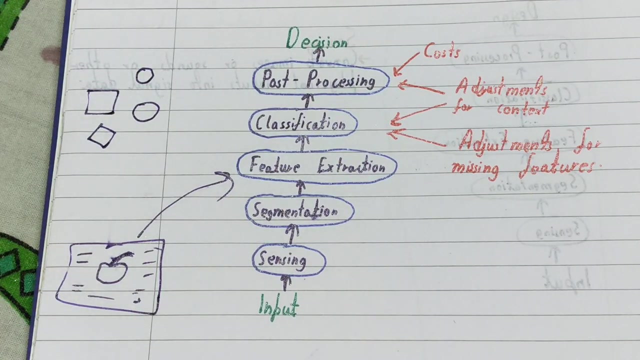 you are provided different shapes and you are asked that how many of them are similar? okay, so here you can tell that this is different, this is a square, this is different and these two are similar. okay, the degree of difference is too much, right, but now let's. it is this and it is. 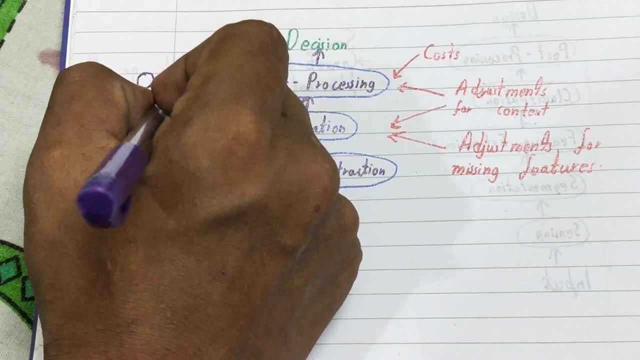 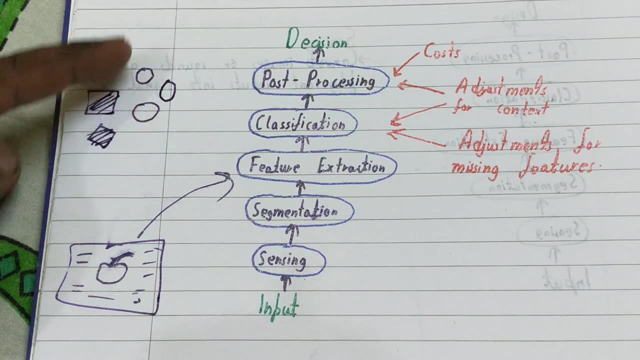 this also. and now let's. yeah. so now you are provided this uh, set of inputs, that is, three similar, look like circles, and you are asked to tell that which of the two are are kept into its same category and which is of the different one. okay, so here you will say that. okay, so this. 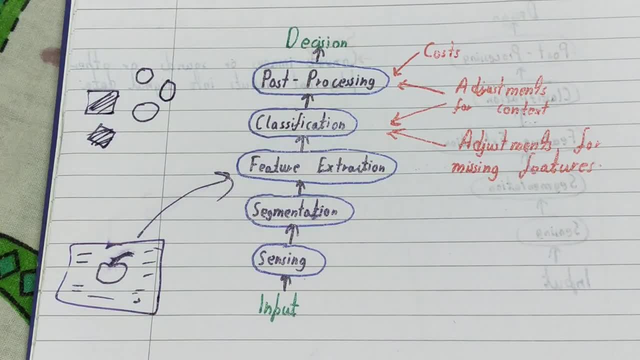 this is also round shape. this is also round shaped and this is also round shape. so if you take a general approach, all of them is kept into the same category. but if you go into a bit detailed one, then you will see that this is a kind of oval shape, right, and this is also kind of oval shaped. so 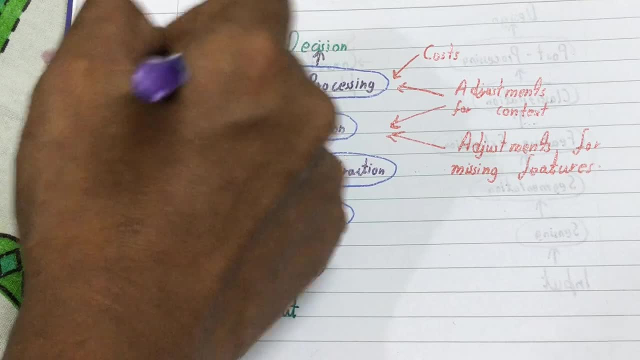 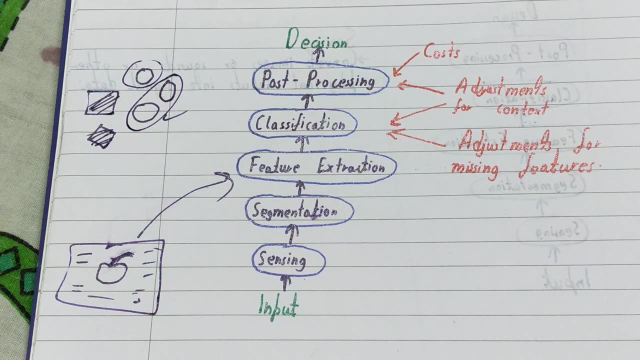 these two can be kept in same category, where this is properly a circle, right? so this can be kept in a different category. so this is how you will characterize, or you can say, classify, a particular object, right? so this is why i say that classification is most important thing that you need to understand, okay? so i guess you are fully clear about. 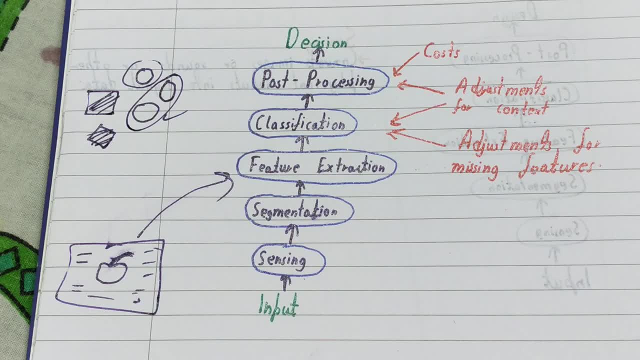 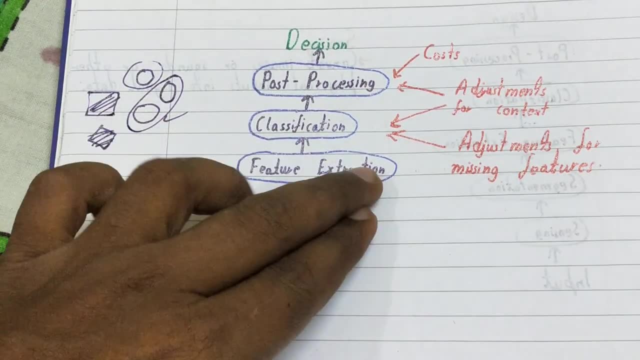 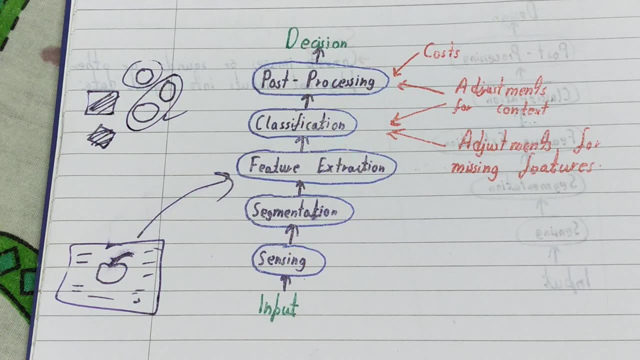 classification- that is first thing, is classification takes full vector data, whatever, whatever feature that are provided for a particular object from this feature extraction stage and it assigns that particular object, a particular category on the basis of that particular features. okay, second thing, the difficulty level that i told you. it depends upon the difference or in the features. 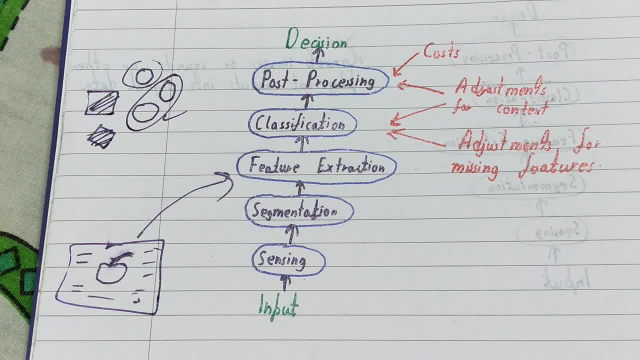 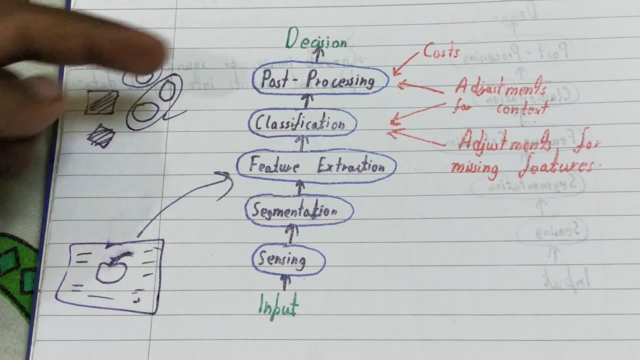 okay, that will. that will determine whether the particular classifier will be easily able to detect or it will be very tough to detect. okay, now let's move on to the final stage, that is, the post-processing stage. okay, so the post-processing component, or you can say the post-processing stage. 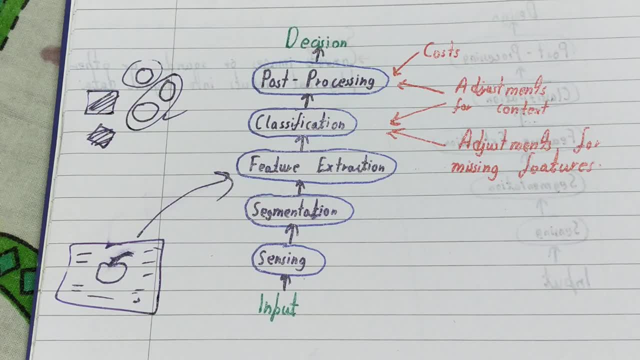 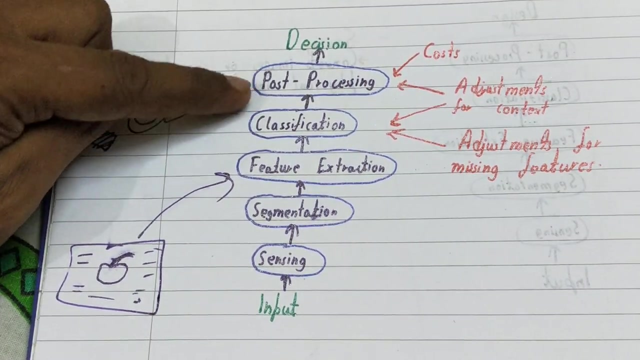 is a very easy stage, okay. so what we do over here is a classic classifier is generally used to recommend action, each action having an associated cost. so what a classifier does is classified, takes out. classifier comes upon a particular decision and upon the decision it advises a particular action. okay, that should be taken by the post-processing unit. or you can say the: 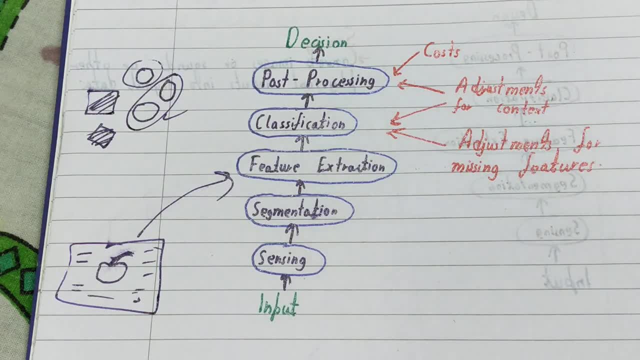 post-processing component. okay, so what post-processing component does is it uses that output of the classifier to decide the particular recommended action. you must be a little bit confused, right? so let me give you a good example again. okay, don't worry. so let me give. let me define a particular set of data. you can use this in your exam as well. okay, 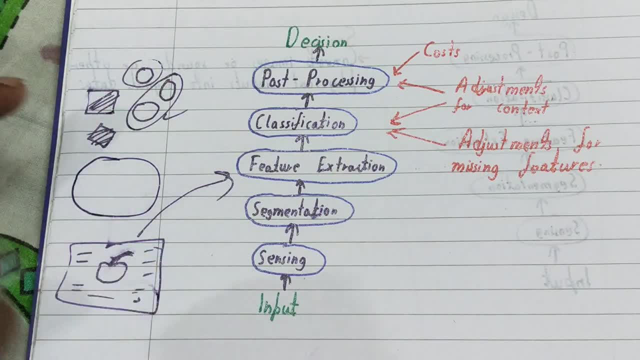 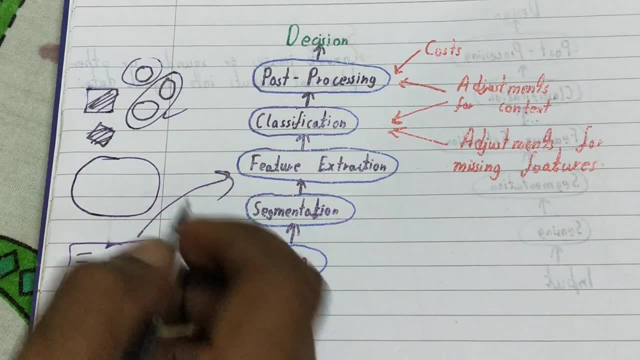 it's not a rough work, kind of you can define each of the stage with the help of this example and writing bit about it. okay, so don't need to worry too much about that. so let me give you a good example here. so let me draw the sample in: 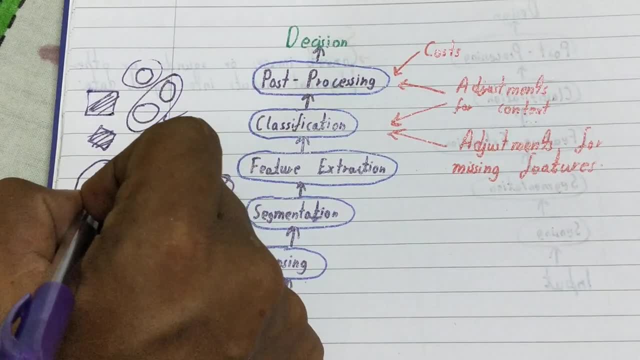 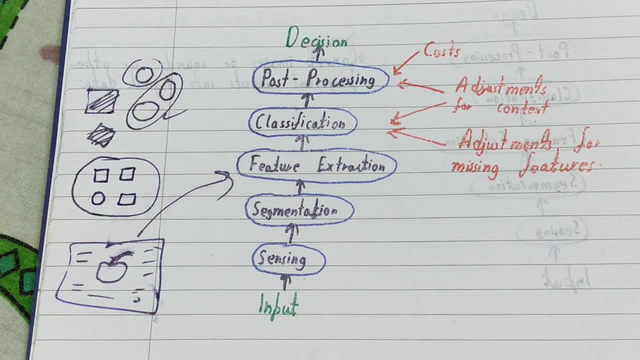 so, for example, you are providing this set of inputs and you are asked to tell that okay, or computer, please tell me the number of rectangles in this set of input data, so the computer will, since each of the data right, then it will sense that this is a particular circle. 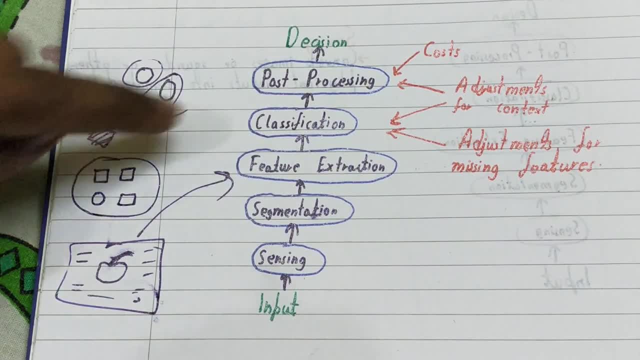 upon coming to this classifier stage, okay, and this will suggest that, no, this one is not a rectangle, and this is an Freddy, or simply factored in by using the vector table. but you can also use a calculator and you can also use a calculator character with the data panel so that also, and in theory, down and connect means to a particular circle. upon coming to this classifier stage, okay, and this will suggest that, no, this one is not a rectangle. I am prepared to give a license before I'll document the part that I am debate them in this, your 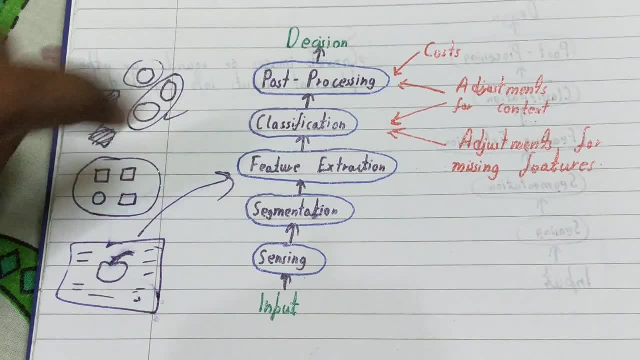 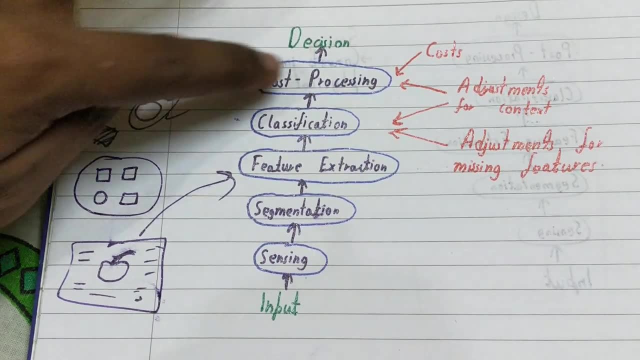 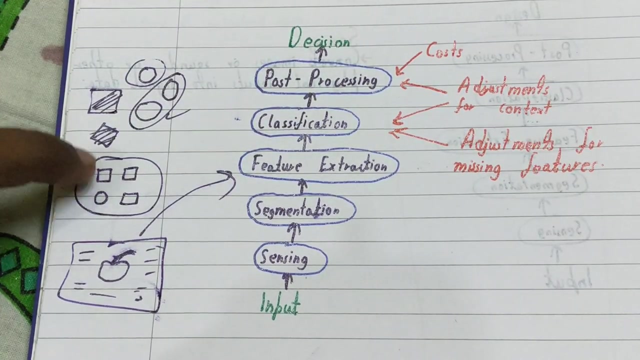 then again it will sense this one, it will come upon this and this will say that this is a rectangle, then declare output that, uh, it has one rectangle. okay, so it will note that. then it will sense this. one same way, same output, two rectangle. then same thing: it will sense again and it will.